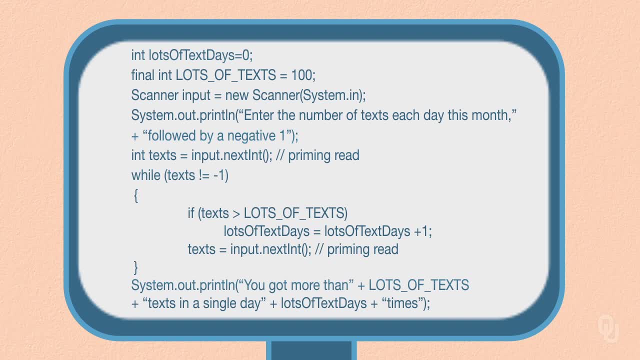 text each day this month, followed by a negative 1. Int. text equals input next int, While text not equal to negative. 1. If text greater than lots of text, lots of text days equals lots of text days plus 1. Text equals input dot next int. System out print line. enter the. 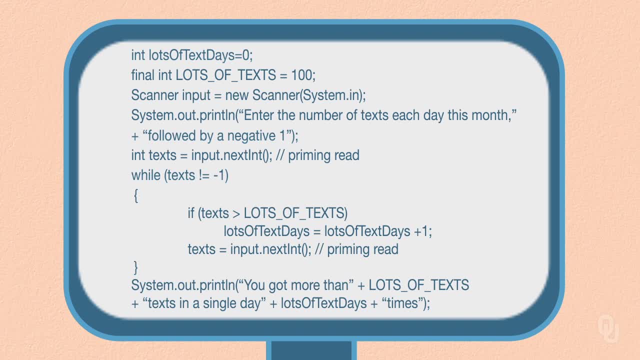 number of text days When you're in core. you don't have to execute any of the functions to use this function. It's just a simple difference in the value of time- The value of time if you're using a standard unit. There are a few things to notice about this code. This code uses a technique that's called 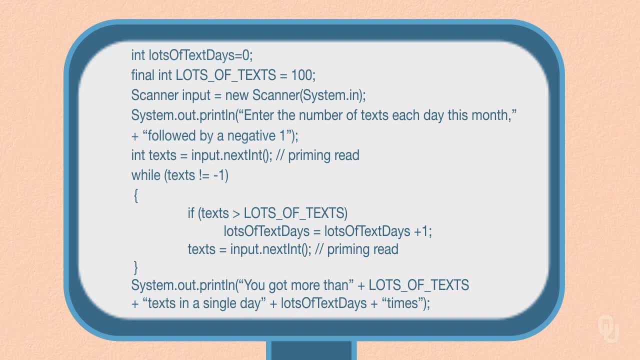 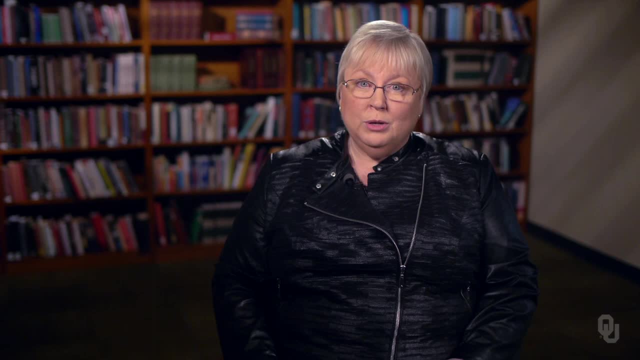 a priming read. I read the first value for text before the loop started. That may look wrong, but it's a logical order when you're dealing with a sentinel, since it would be possible that someone would enter the sentinel value first. In that case, the loop wouldn't. 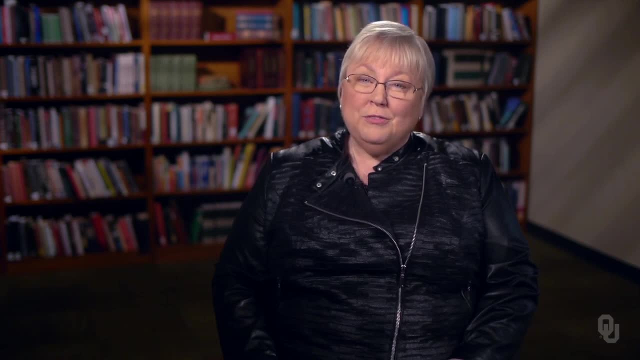 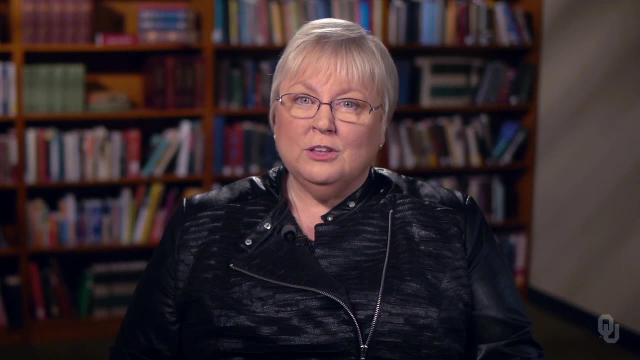 entered at all and the correct results would be shown. The value for the second iteration of the loop is read at the end of the first iteration. The reason you do this with a sentinel is that you want to exit the loop immediately when the sentinel has been entered. If you're wondering why we call this a priming, 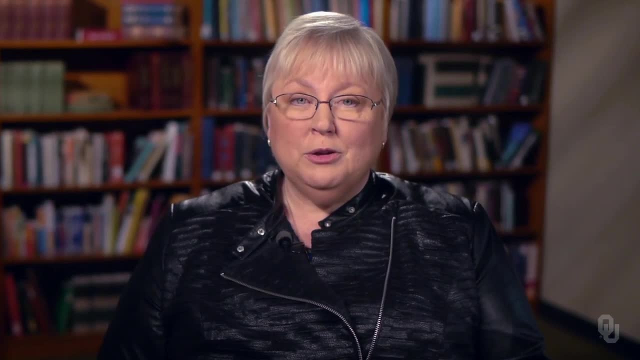 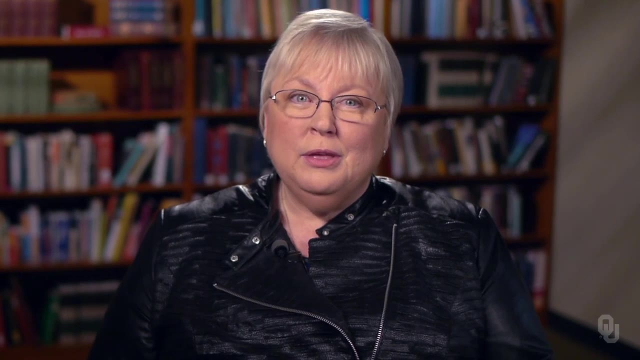 read. it's similar to priming a pump. If you've ever had to pump water from a well manually, you probably know that you sometimes have to pour water down a pump. to pump water up The read before the loop is like pouring the water down the. 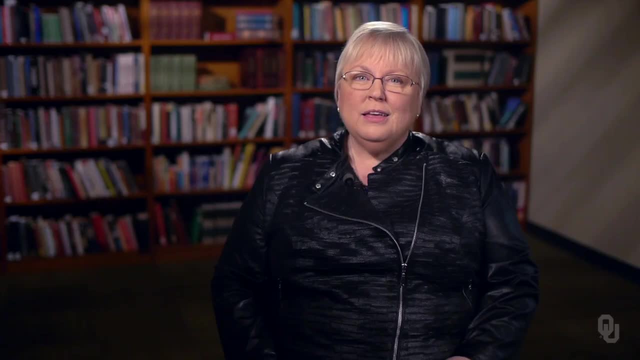 pump. I admit the analogy isn't perfect. Nesting is a profound idea of computer science. You've seen nesting before. if you store files and folders on your computer, Folders contain files and other folders and those folders contain files and other folders, and so on. The fact that a folder can contain a folder and 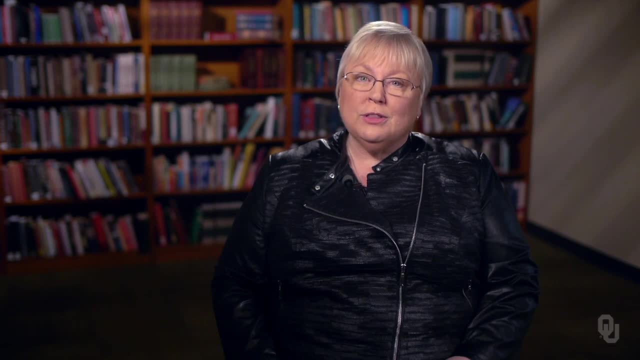 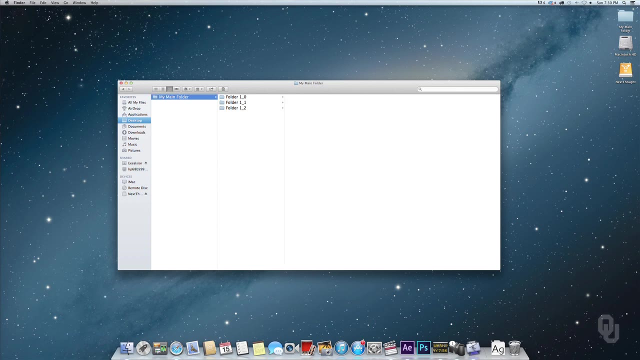 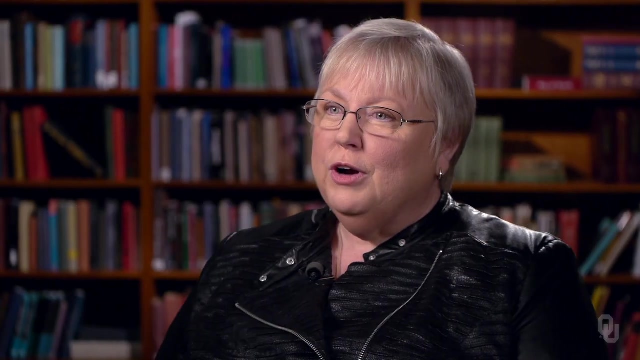 that that folder can contain yet more folders is a particularly elegant example of nesting. This shows up really nicely on a Macintosh computer, where each layer of folders is in a vertical list and moves left to right as the folders are open and closed. Another way we can improve our use of control structures is to 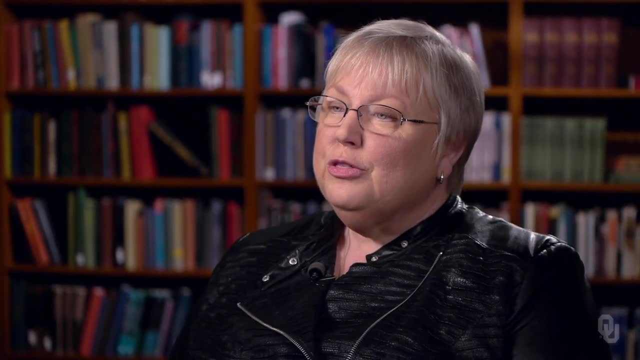 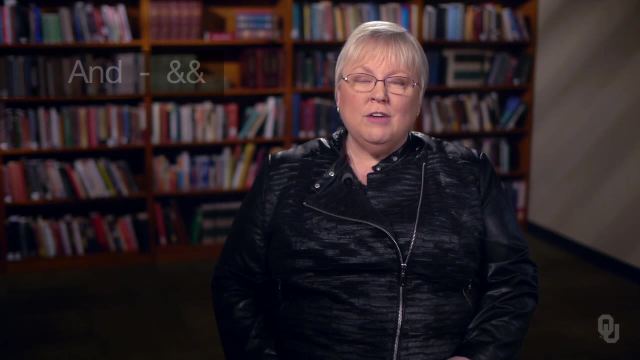 learn to combine boolean variables together. There are three essential operators for boolean variables: and or and not. The symbol for and in Java is a pair of ampersands. The symbol for or in Java is two vertical lines. The vertical line key is usually on the right-hand side of the keyboard, above the 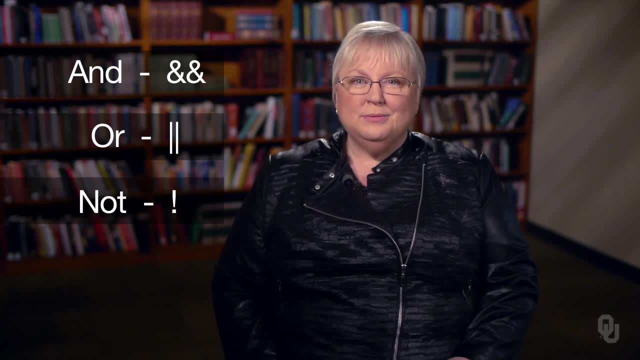 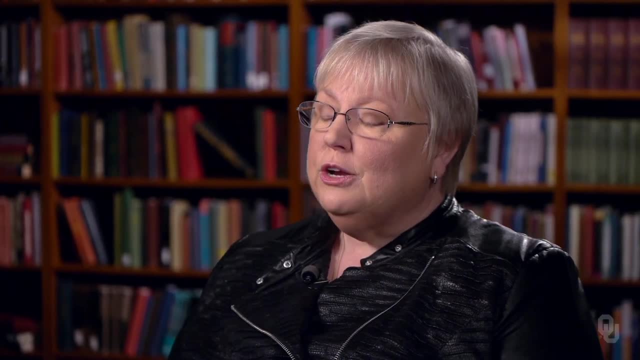 enter key, Not is an exclamation point. While we use these words in English all the time, their computer science meaning is much more precise, particularly with or If I say I'm going to the store or picking up burgers, you'd probably be. 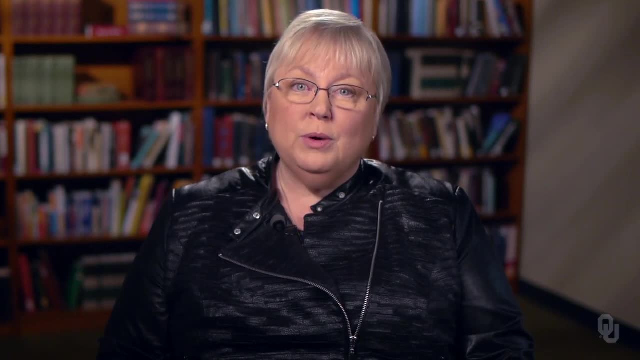 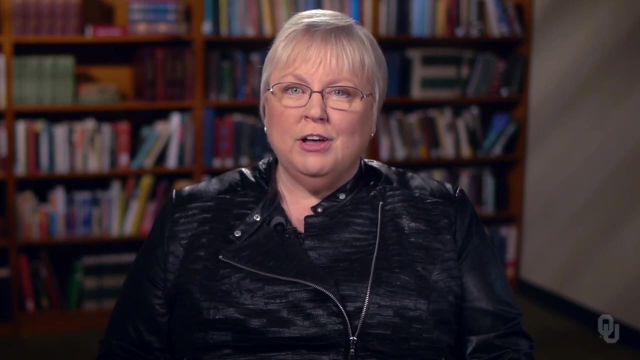 surprised if I did both. But in Java, or is true? when either one or both of the booleaned operands are true, The and operator works pretty much the same in in English and Java, as does the not operator. Suppose we want to count the number of words. 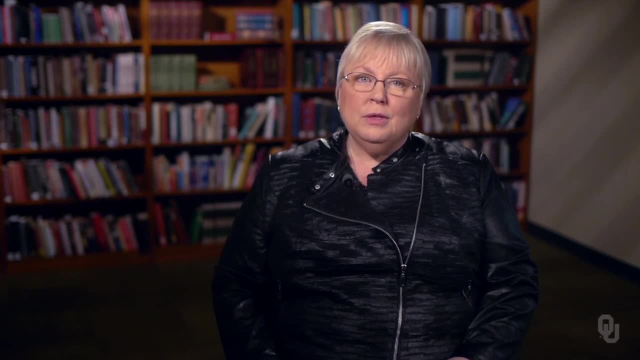 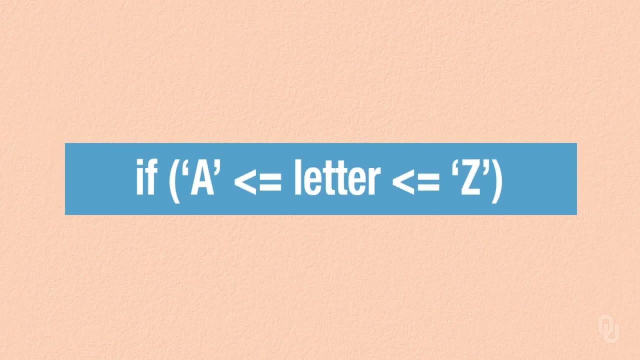 in an array list of strings that start with a capital letter. You might think we could do something like this If a is less than or equal to letter which is less than or equal to z, but that doesn't work in Java. The problem is that a less than or equal to letter is: 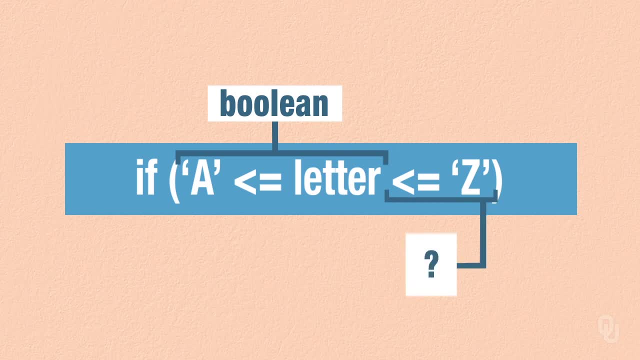 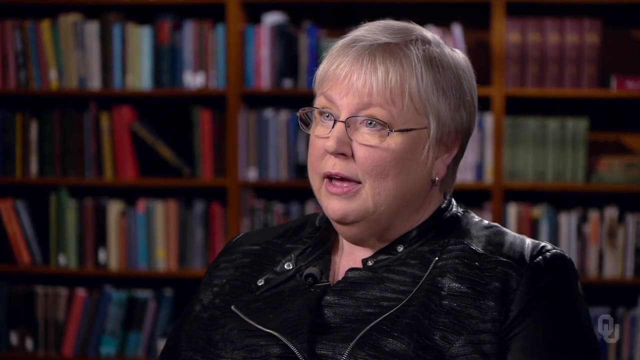 a Boolean and true less than or equal to z doesn't make any sense. So we have to use logic operators to combine the test of whether the letter is bigger than the character capital A and the letter is smaller than the character capital Z. Let's look at some code: Int count. 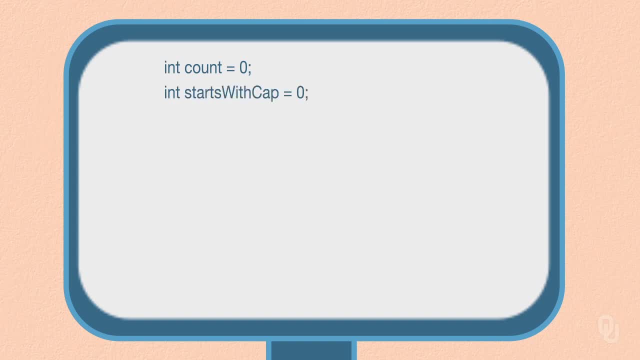 equals zero. Int starts with cap equals zero. ArrayList of string list. Let's assume this list is constructed and data was entered elsewhere. While count is less than list dot size. char letter equals list. dot get of count. char add of zero. If a is less than or equal to letter and letter is less than or equal. 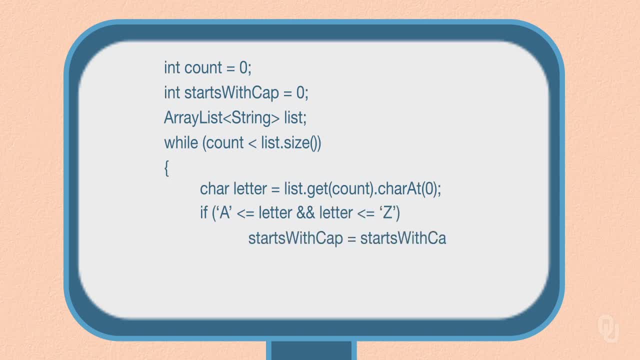 to z. Starts with cap equals. starts with cap plus one. Count equals count plus one. This code steps through the ArrayList of strings, named list, one element at a time. It takes the first letter off the string and stores it in letter. Notice that I have two dot operators. 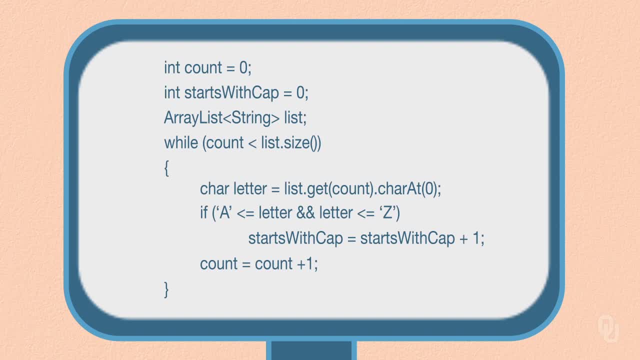 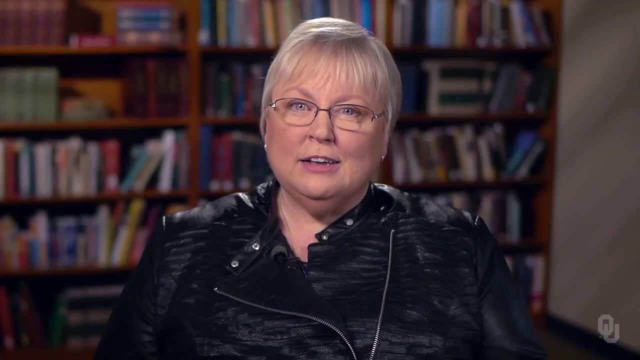 together on one line. The left dot operator applies to the list and the right one applies to the string that's returned. The left dot operator is returned by the list dot get method. If you find that syntax confusing, you can pull the string out of the list in one step and store it in a variable Once. 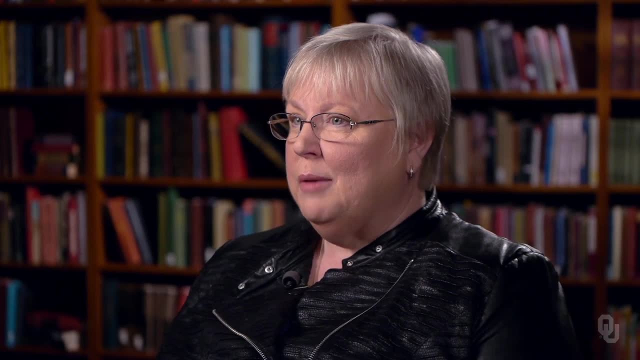 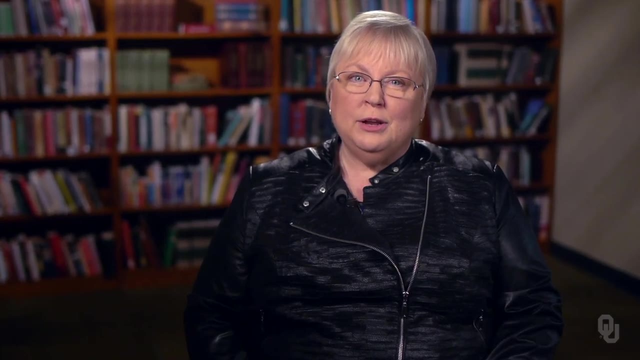 we have the letter, we can test to see if it's between capital A and capital Z and increment the counter. if it is Now that you know how to nest control statements and use logical operators, we'll be able to create bigger and better programs.